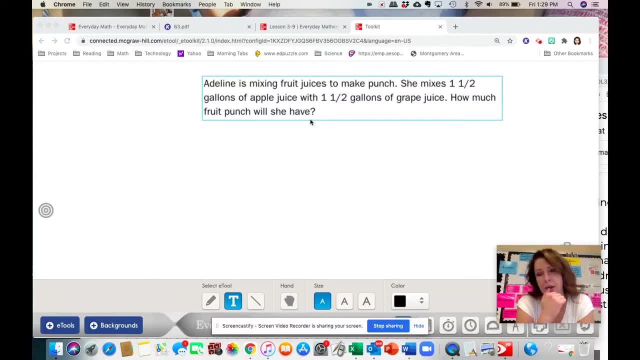 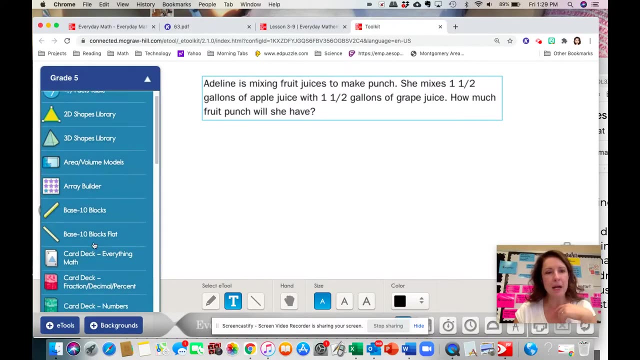 So when I think about how I could solve the problem- fractions, mixed numbers- I tend to think of fraction circles. So I'm gonna use fraction circles to prove this answer and to confirm my estimation, because I can look at those two and I can estimate where I believe them to be. 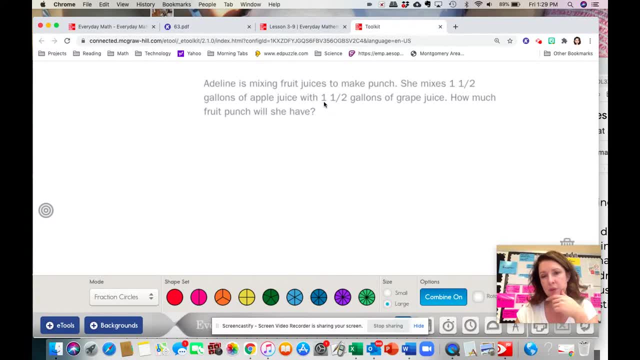 because I am confident with my ability to look at halves and put them together. But just to prove it, we're gonna pull up some fraction circles. So she starts with 1 1⁄2, and then she she gets another 1 1⁄2.. 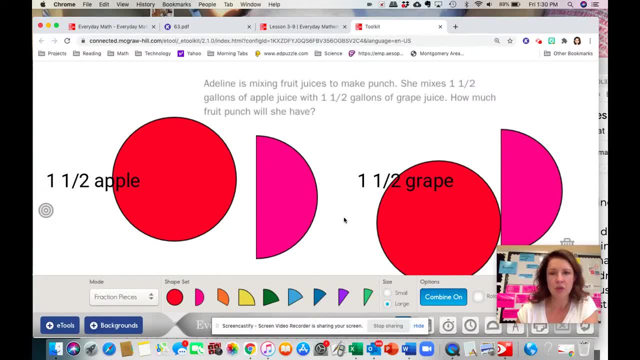 So there's my representation of the apple juice and the grape juice. So now I need to solve it by putting them together. So I'm gonna take this one over here and prove my answer, which is what I was predicting and estimating it to be. 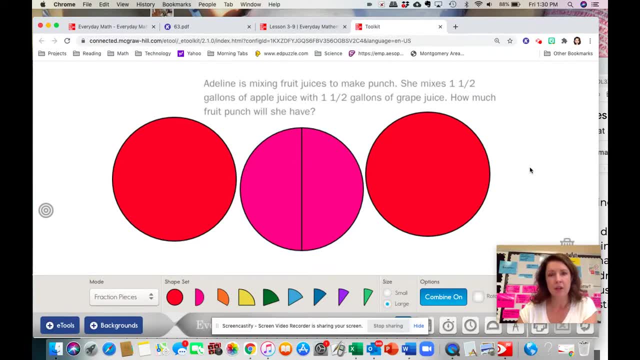 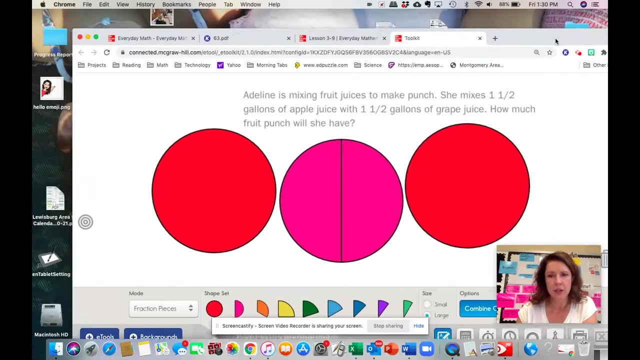 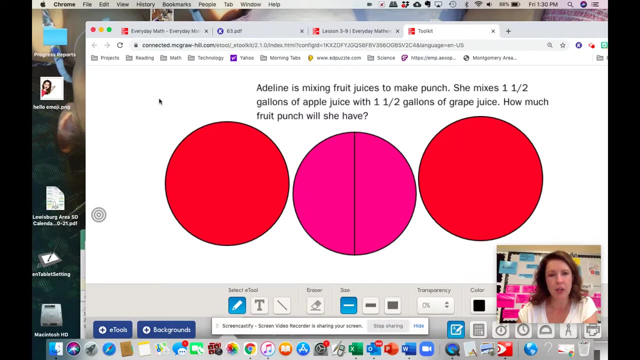 which was around three, and it is indeed three. Finally, what do we label it? Three gallons, Three gallons. So, going back to my problem-solving strategies, I definitely, when I'm reporting my answers, wanna make sure that I've double-checked. 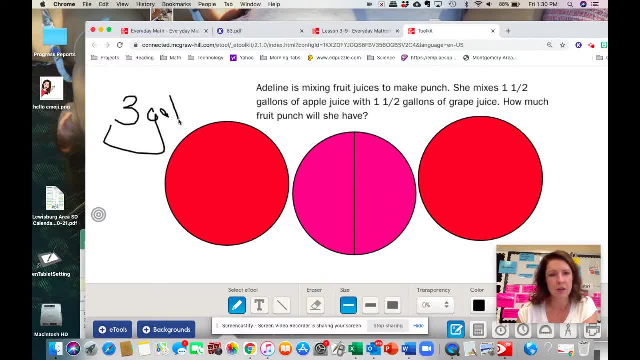 and make sure I've labeled correctly: Three gallons. All right, so let's take a look at another problem, this time from your math journal. So if you have your math journal handy, you can go ahead and type in your math journal. 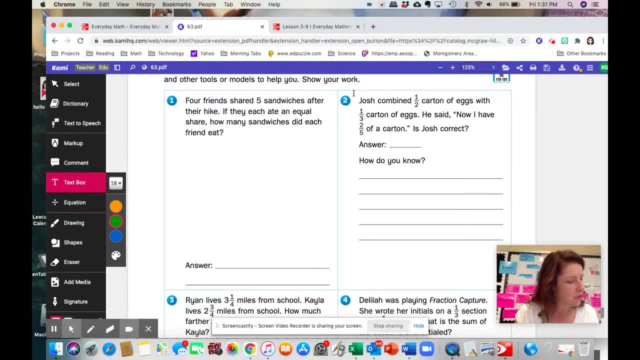 So if you have your math journal handy, you can go ahead and type in your math journal And could go to page 101.. This is problem number one. So we're looking at four friends sharing five sandwiches after their hike If they each ate an equal share. 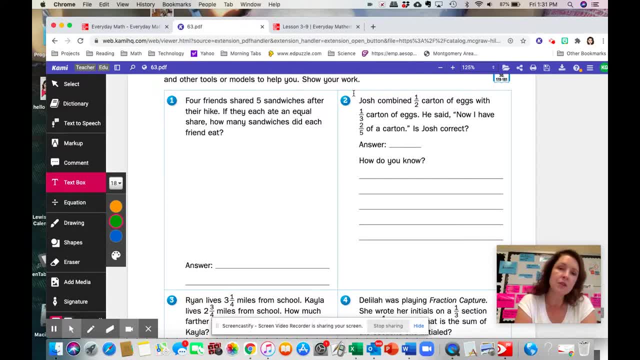 how many sandwiches did each friend eat? So as soon as we start looking at equal shares, we have to start thinking about division, dividing up an item to share amongst people or objects Or containers. So in this one we have to think about 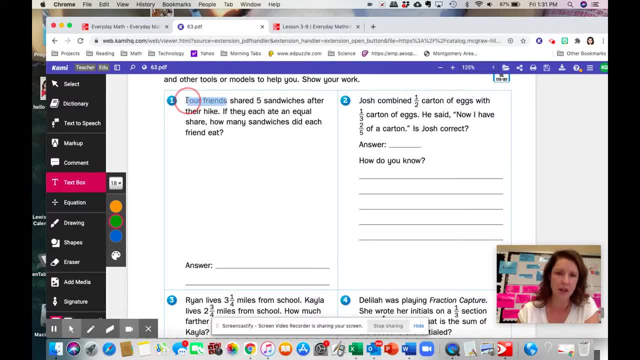 what is the thing being shared? Well, we're not sharing the four friends, We are sharing the five sandwiches. So I do recognize that this is the thing that needs to be shared And who is sharing it? It just says that there are four friends sharing. 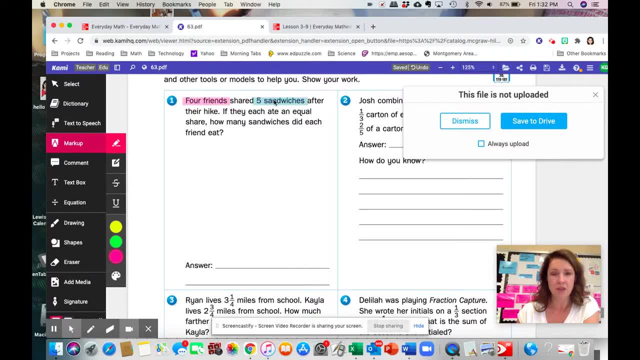 So I do recognize that four friends have to share five sandwiches. So I could draw a picture, I could write a number model, But ultimately my end goal is I need to figure out how many sandwiches each friend ate. So I'm gonna do, I think, both. 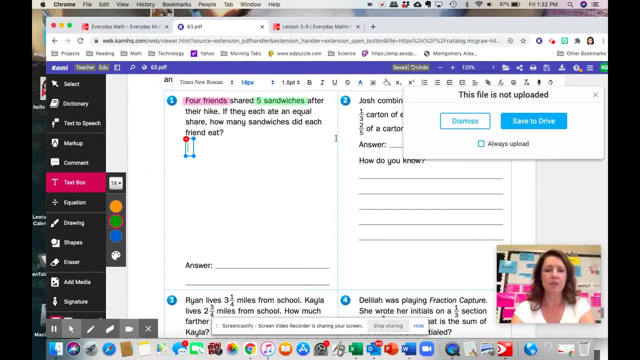 I'm going to put a number model in: Five sandwiches are being divided amongst four friends, So that will give me what. And then I'm gonna do an illustration because again I've made an estimate in my mind that they're each going to share five sandwiches. 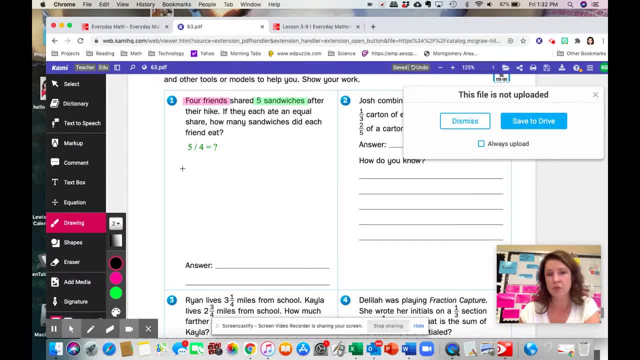 I'm going to get at least one, but then I'm not sure of how much more they're going to get, So I'll go grab my shapes and we'll get some sandwiches here. Okay, so there's my five sandwiches And my people. I'm going to make my people below. 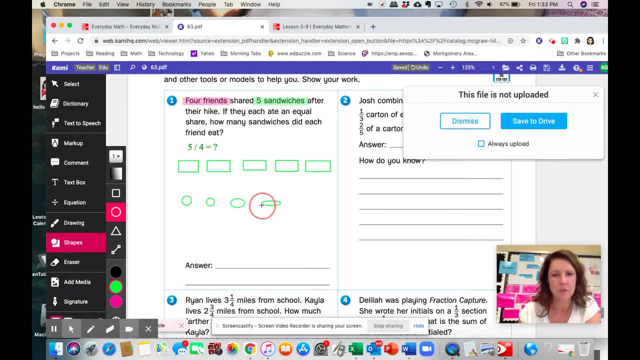 Okay, there's my four people. I can help them out a little bit and give them a body. Okay, so my people are going to share. So I could either break all the sandwiches up into fourths and then count up how many fourths there are. 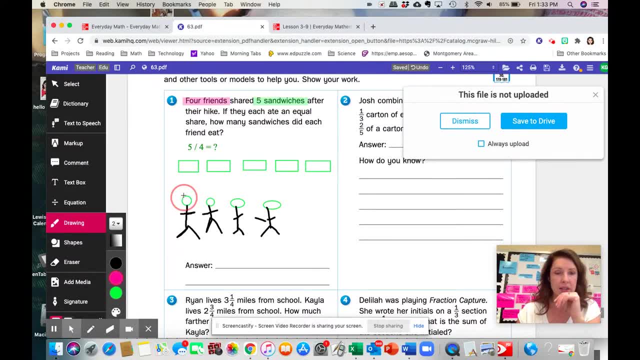 or what I think would work better is. I can just say that person one is going to get this sandwich, person two is getting this one, person three is getting this one and person four gets this one, which leaves only the last sandwich to be broken into four pieces. 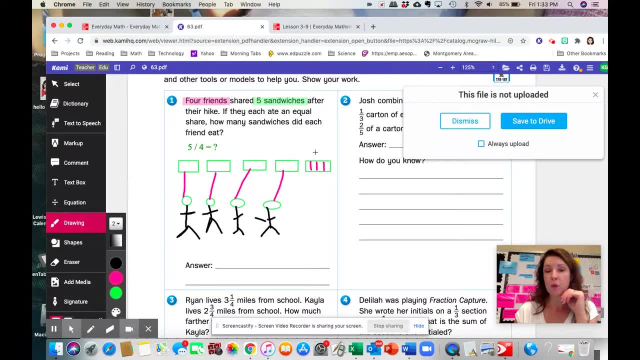 So because that last sandwich has to be shared and it's broken into four pieces, my denominator will be a four and each person will get one of the pieces, giving us one fourth. So my answer is that each person gets one and one fourth sandwich. 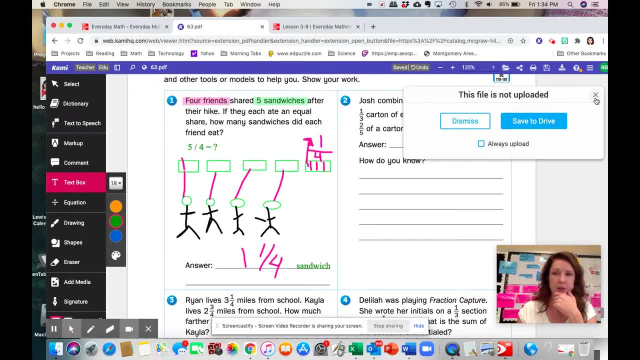 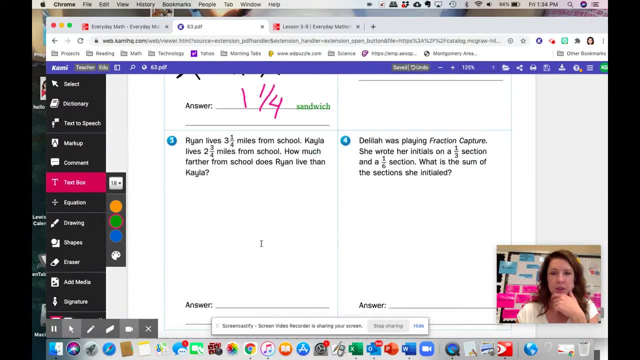 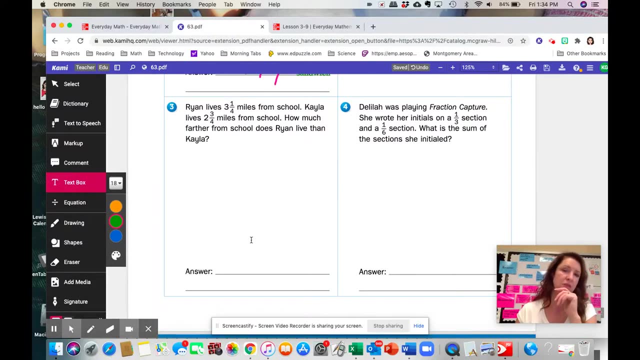 Okay, Moving along. So let's take a look at number three. Ryan lives three and one fourth miles from school. Kayla lives two and three fourths miles from school. How much farther from school does Ryan live than Kayla? So how much farther? 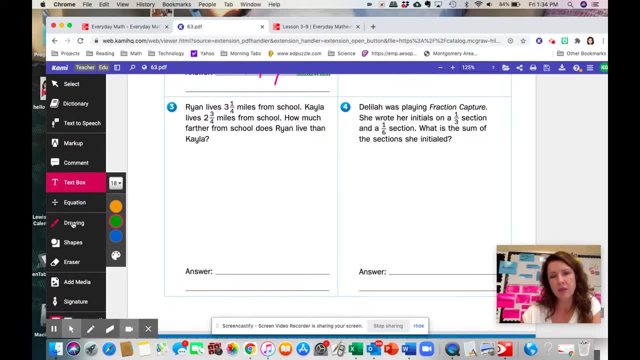 Well, I know I need to figure out distance, and it's in miles, And I know when it's talking about how much farther we're looking at removing, we're looking at subtracting. So if I want to illustrate how much farther I live, 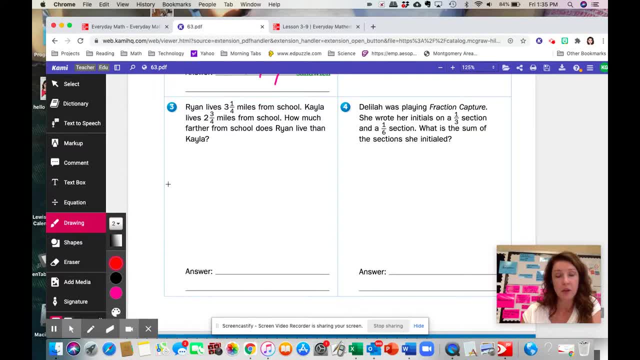 I'm going to have to break it up into four parts. So if I want to illustrate what's really happening, I could draw a number line- zero miles and four miles- And I could break it up: one, two, three, one mile, two miles, three miles. 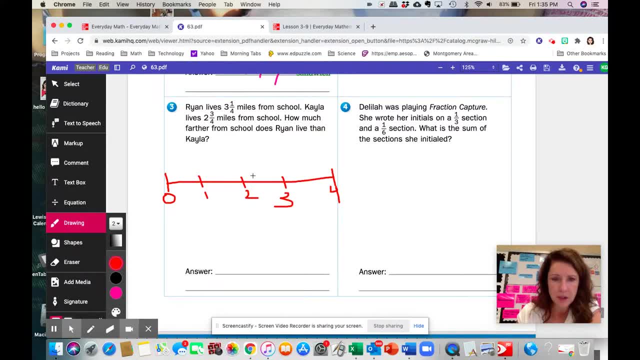 And because the denominator is fourths, I'm gonna have to break them into. I'm gonna have to break a whole into fourths. So I'm gonna do that with the last two wholes, because I don't really need to break these up yet. 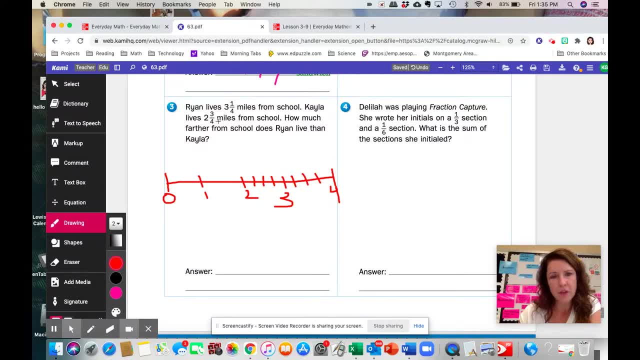 because this is where I'm starting. I'm looking at three and a fourth and two and three fourths. So Ryan lives at three and one fourth mile from school. So on the number line he is here Three and a fourth And then Kayla lives two and three fourth miles from school. 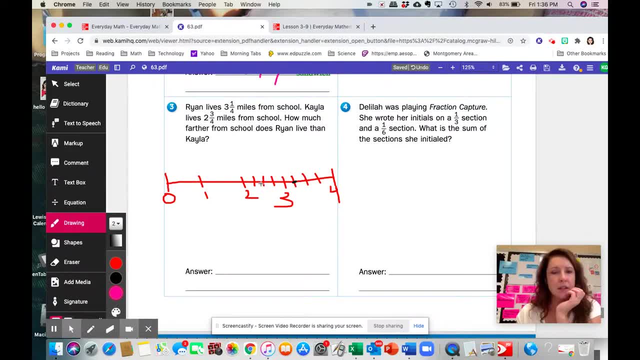 Kayla, let's go make her purple. She's here. How much further does Ryan live than Kayla? So he's here The school's way back here School And if we go back one, two fourths, he lives two fourths miles further from school.